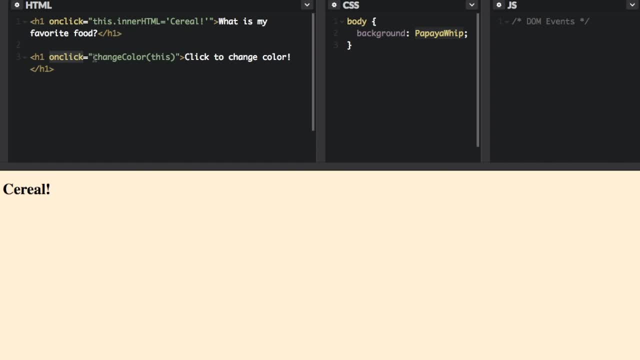 code. So if we have the onClick event we can call change color and then pass in this. that means we're passing in this h1 tab, we're passing in this whole thing here to the change color function. So over in the JavaScript. 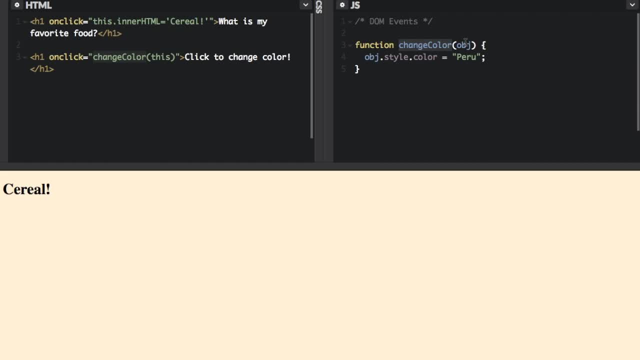 section. we're going to put this change color function. it's going to take an object And then we're gonna do object dot style, dot color equals Peru, because Peru is not just a country, it's a color also, at least according to your browser. 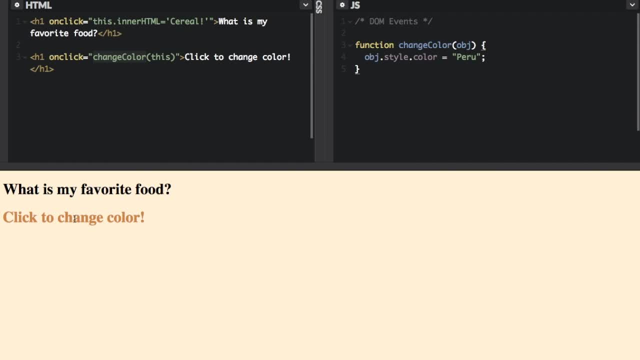 So reset this. if I click here, it's now changed to the color Peru. Now, on these two, we set the on click event right in the HTML. However, you can also set the on click event in the JavaScript. So here's a button here And there's nothing in this button that shows what happens when you click the. 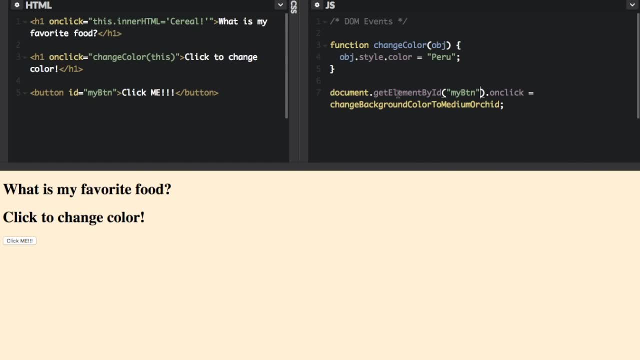 button. But over in the JavaScript I'm going to put in some code here. First we're going to get the element document dot. get element by ID. my button, that's this button over here, And then we're going to set. 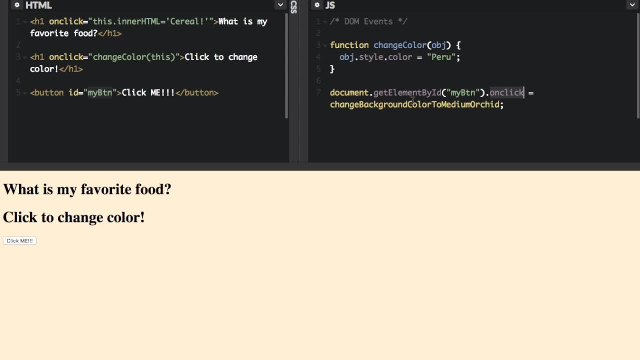 an on click event right in the JavaScript And the event is set to change background color to medium orchid. Now this is just a function call that we now have to create. Okay, here's the function function- change background color to medium orchid- And we're going to do document that. 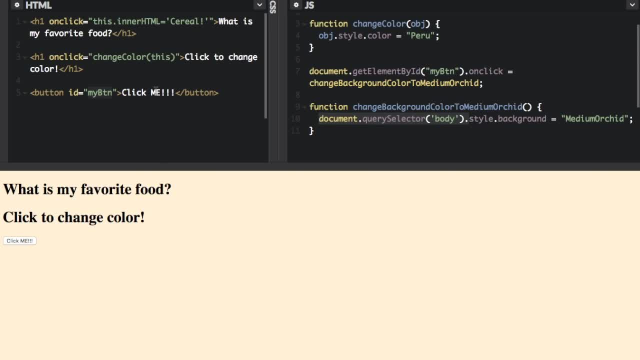 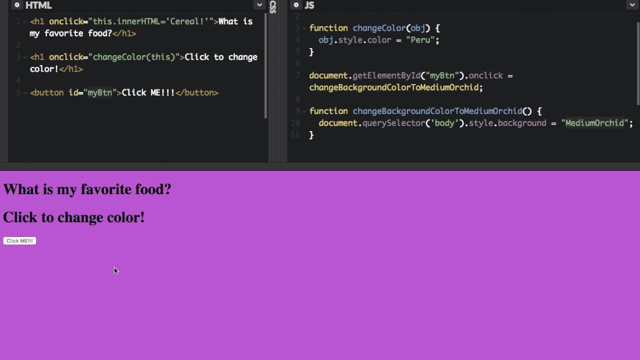 query selector body. So that's going to apply to the whole body of the HTML And we're going to set the style dot background to mean orchid. meeting market is another color In your browser. if I click the button here, it's medium orchid for the background. So that's how you can. 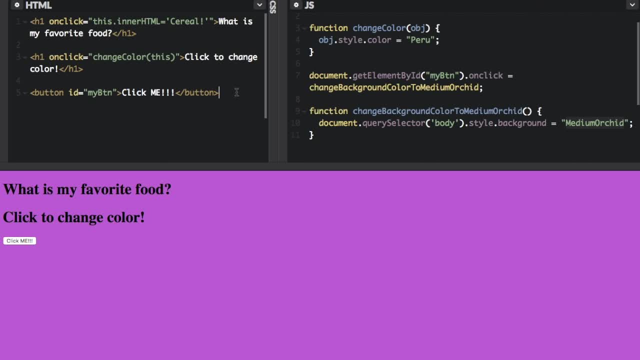 change the background of your whole page. Besides on click, you can also use on load or on unload, So that would be something like this: you would normally put it on your body tag, which would be at the beginning, and code pin. you don't use a body tag, But if you put an onload event on your body and 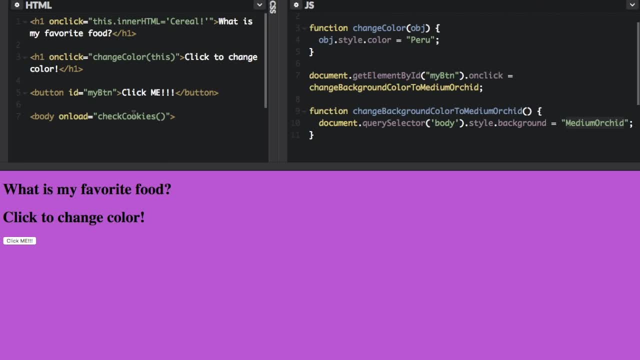 you run a function here. these events are often triggered when the user leaves the page And they often are used to deal with cookies when you're just using the onload and on unload. But we're not going to use this right now. So another thing I wanted to show you is on. 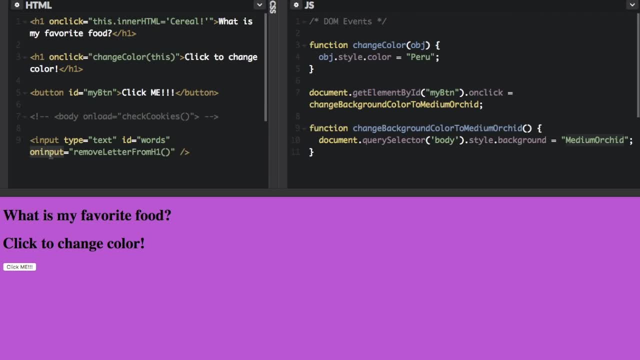 input. Let's bring this down a little bit on. input means: whenever you input any characters or anything, it's going to call function here. So here we have the text box down here. And now every time I put in any letters calling a function, I created the function Yes. So now it's not doing. 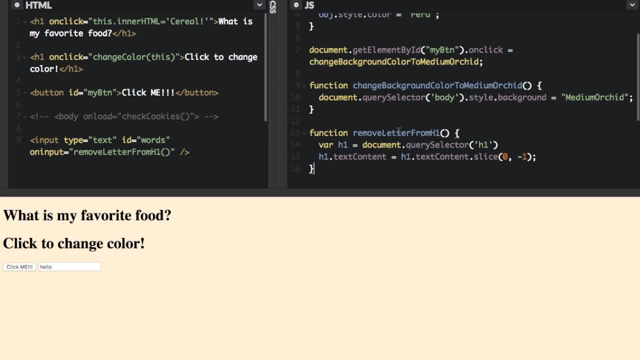 anything. So let's create the function here. So let's create the function here. So I'm going to create that function. So the function is: remove letter from h1.. So we're going to set h1 variable to document that query selector h1, that's just going to select the first h1 tag on the HTML page. 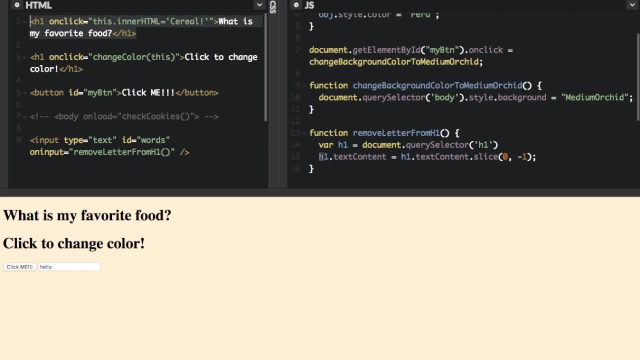 which is this one up here. Now we're going to find the h1 dot txt content. That's the text inside the h1 right here, What is my favorite food? And we're going to set that equal to h1 dot txt content. So we're saying that, setting equal to itself, but then we're slicing it passing. 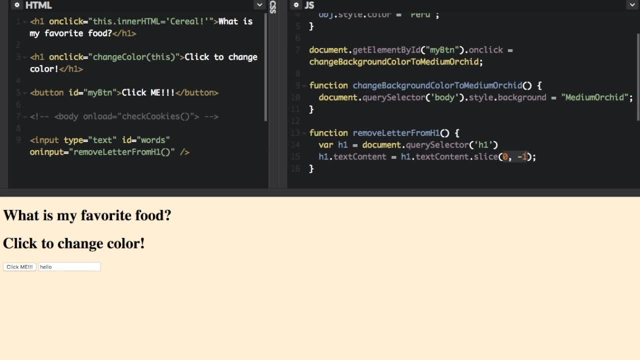 zero negative one. that means we're just taking off the last letter of that field. Now, this whole function is kind of just for fun, just to see what you can do. So let's see how it works. As you can see, every time I type a letter, another letter from the h1 tag gets removed, Also interestingly. 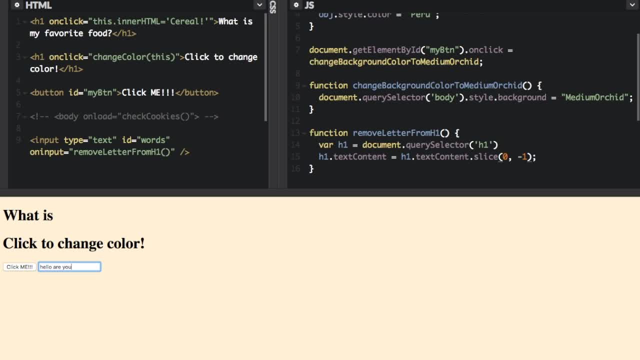 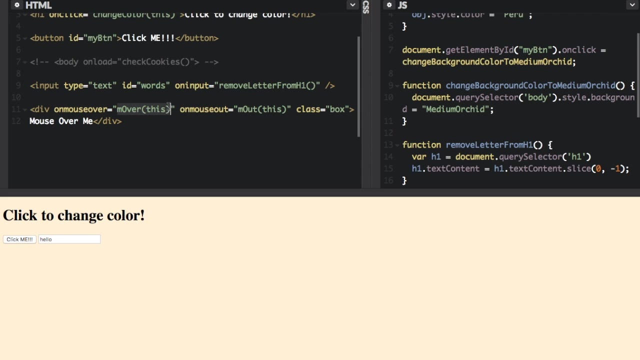 anytime I delete a letter, something is removed too, because I'm putting an input of delete and it's still removing letters. Oh, the whole text is gone. And let me show you some other events. you can do So here. I have a div And there's an on mouse over event that calls this function here. 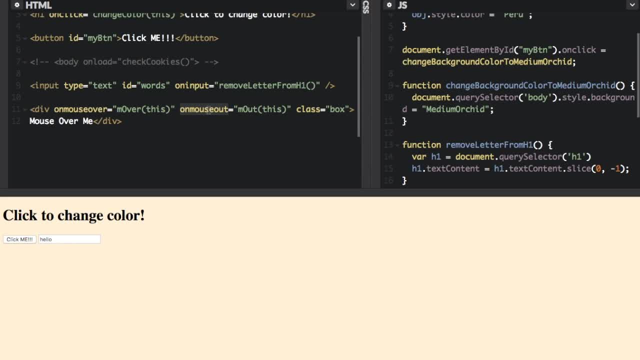 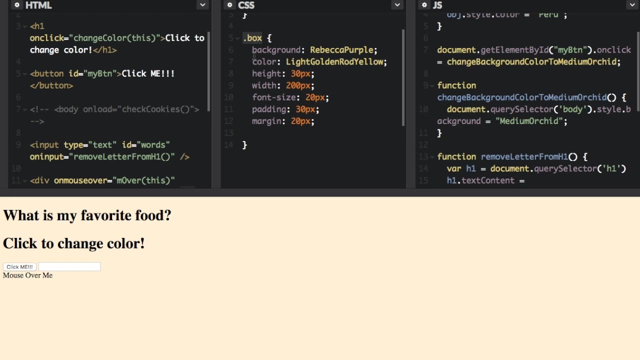 and it passes in the div. And we have an on mouse out event that calls the in out function and passes in the div again and we have a class of box. So let me put some CSS in here to make it look how we want it to look. So dot box just means we're setting the class box. 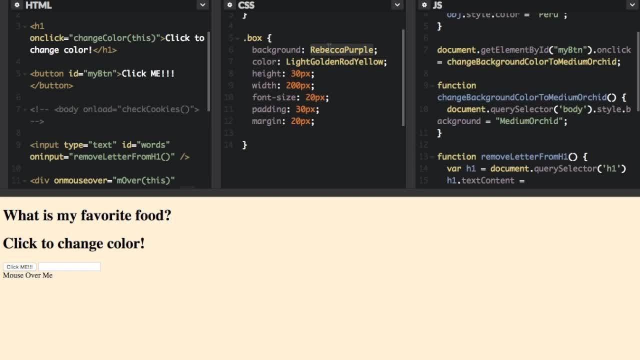 To have these things for background, we're using the color Rebecca purple, So for some reason Rebecca gets her own purple, And then the color of the text is like goldenrod yellow- one of the longest text names- And then we're just going to set the height and the width, the font size and 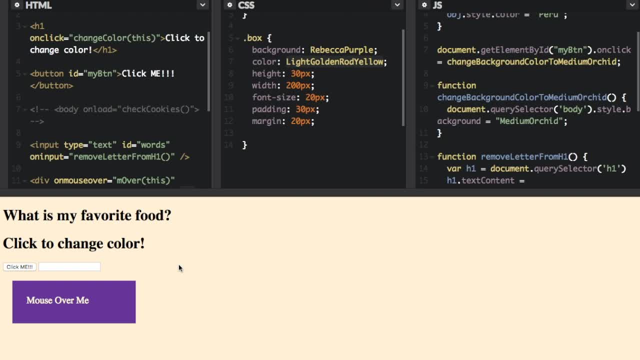 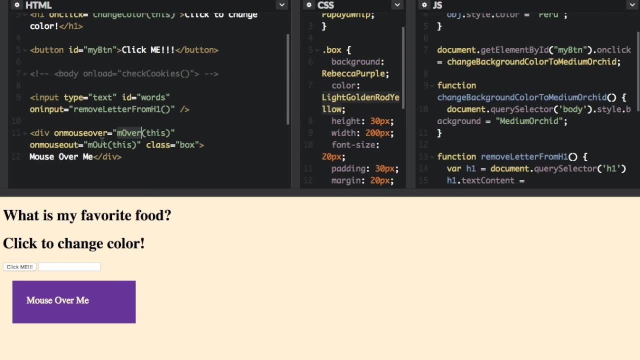 some other things. So let's see what that looks like. And there's the box, And right now, if we mouse over and mouse out, nothing happens. So let's create these JavaScript functions, the M over and M out. Okay, here's M over and we're receiving the text, And then we're going to do a.